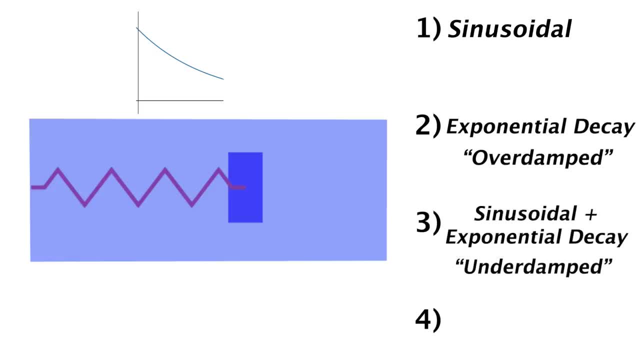 Three is a combination of the first two, which happens when the damping isn't as strong or the spring itself is stronger. In this case, the spring will oscillate but still decay in the process until it eventually settles. And four, literally anything else can happen if we have some input force or just non-ideal. 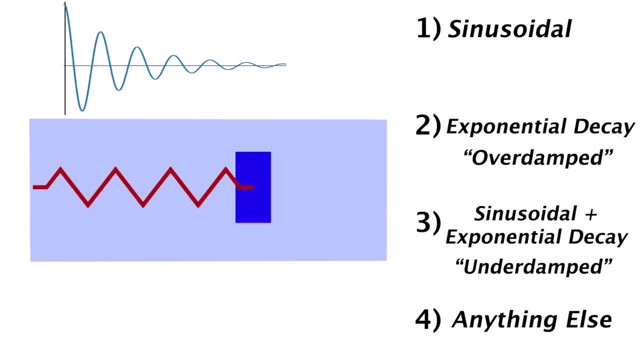 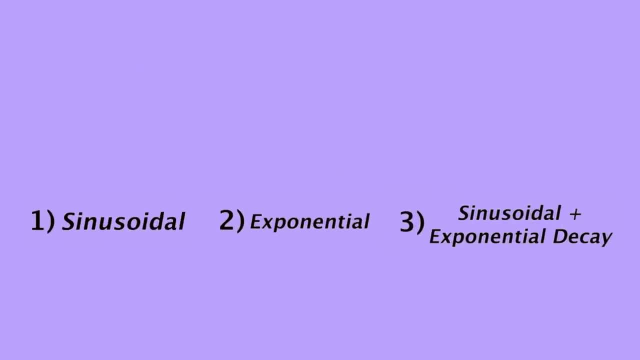 conditions. We're not directly as concerned with this fourth case in this video, but we'll get to that in a minute. So let's get started Now. if I had to summarize what the Laplace transform visually tells us in just a few seconds, it'd be this: While the Fourier transform tells us which frequencies or 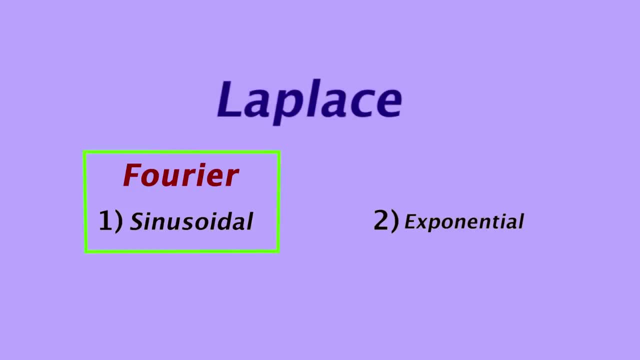 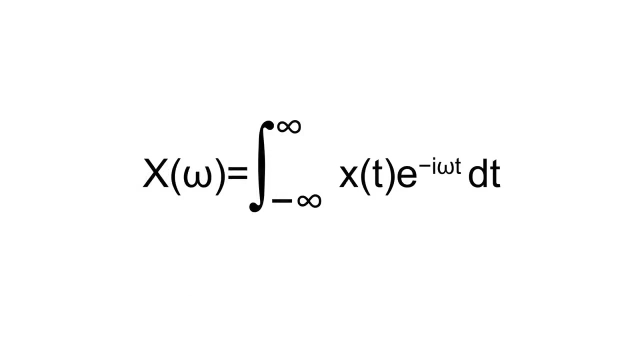 sinusoids are present in a function. the Laplace transform tells us which sinusoids and exponentials are present in a function. In fact, we're soon going to see that the Fourier transform is just a slice of the Laplace transform. Now here's the Fourier transform equation. It takes in some function. 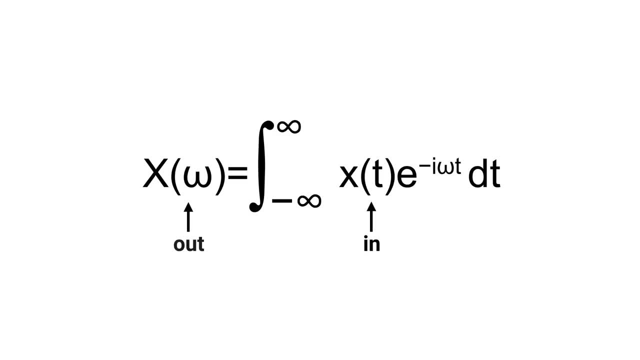 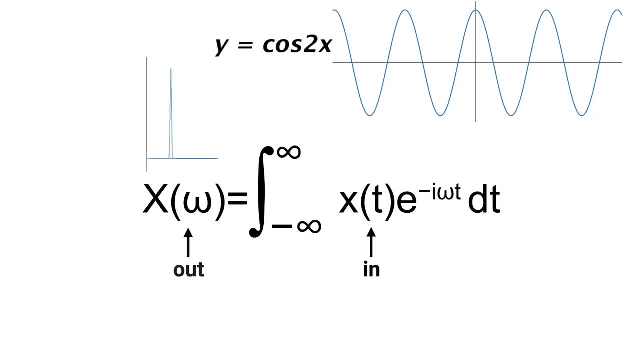 of time and outputs a function of omega that tells you which sinusoids are present in your signal. If you put in a pure cosine curve, then out comes a function with one spike, since the original curve was one sinusoid. Well, for real functions these are symmetric about the y-axis, so you'll. 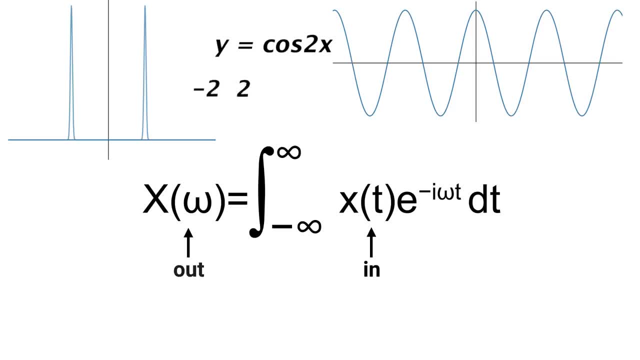 actually see two spikes And the x-coordinates will match the angular frequency of the original signal. If you put in a non-periodic function, you'll get out something more complex which tells us that it takes infinitely many sinusoids to make up this function. on the right. 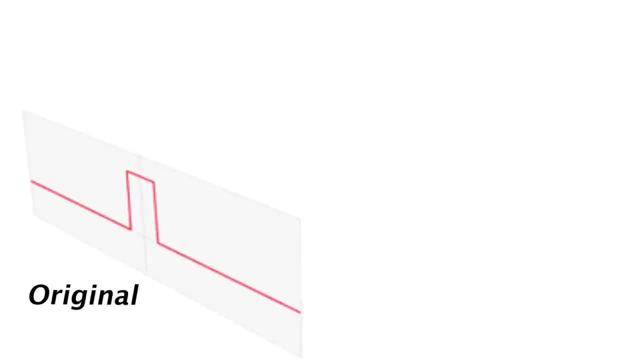 This animation does a great job at showing the original function being a sum of all those sinusoids, infinitely many, where the sum is seen in yellow, while the magnitude of the Fourier transform tells us relatively how strong each of those sinusoids is for any given frequency. 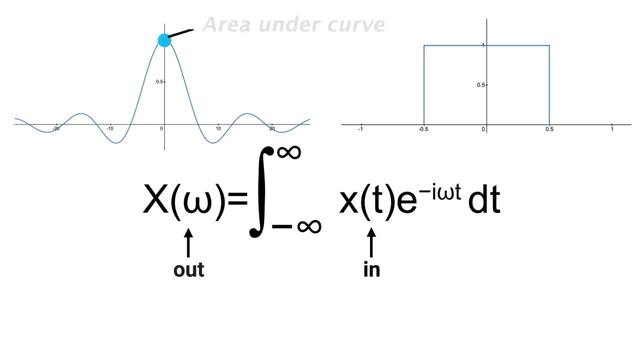 One thing to note is that the y-intersection has a maximum value of n. intercept of the Fourier transform is the area under the curve of the original. Remember, this is the output when omega equals zero. And when omega equals zero, then this term goes to one and we have just the integral of the original function. 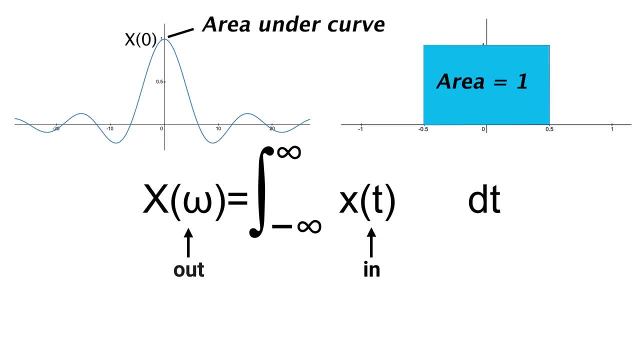 aka the area under the curve. Now for a lot of this video I'll be working with this equation or something similar, because it has a sinusoid and exponential component. However, we will assume it's zero for all negative values of t and it essentially turns on at time equals zero. 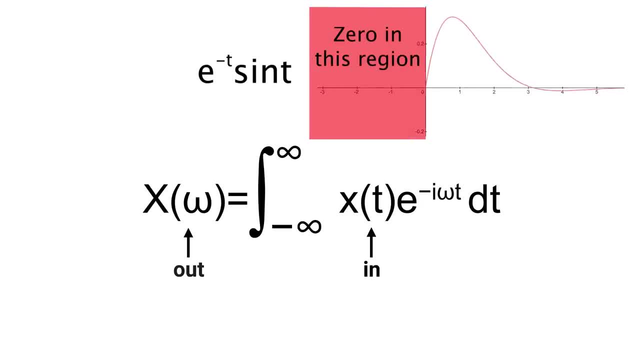 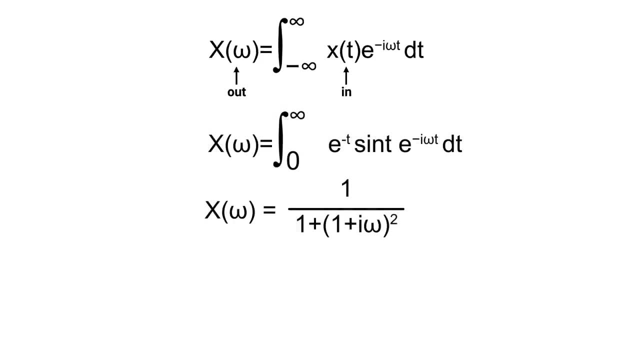 which avoids the function diverging to infinity. So when we put it into the Fourier transform, out comes a complex function that I won't graph quite yet. I'm not worried about the calculus in this video, but if you just know integration by parts, you can do this. Just treat i as a constant. Anyways, I'll foil the bottom here. 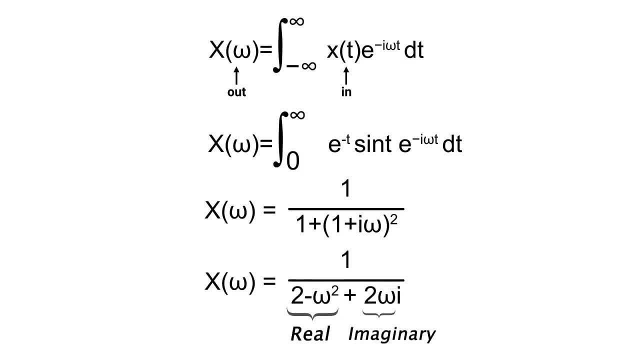 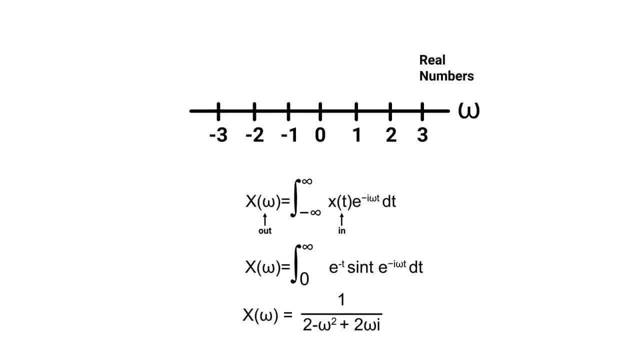 to get a new equation, just with a separated real and imaginary component, and this is what we'll work with. This function only has one input, omega, so that can just go on a number, but out of the function will come a complex number with a real and imaginary component. 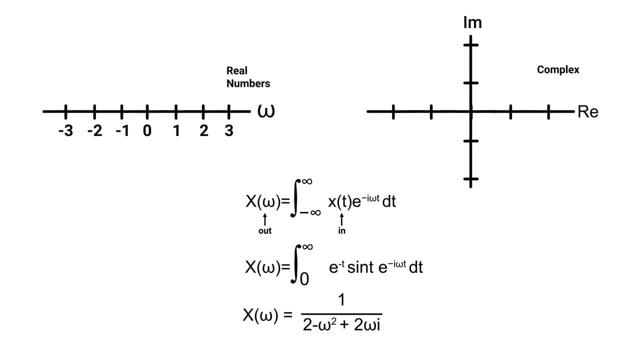 so we need two dimensions to represent that. So let's put in some values now. If omega equals one, then the output becomes one over one plus two i, but that can also be rewritten as 0.2 minus 0.4 i. 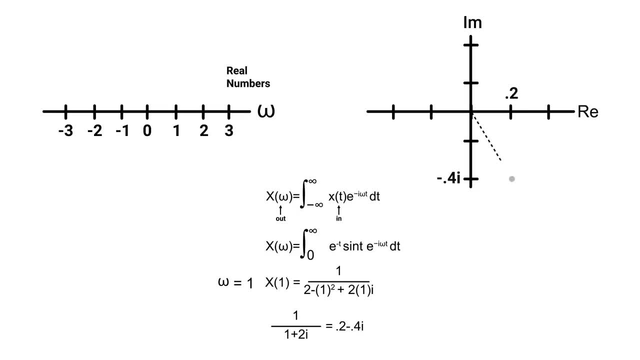 which will be plotted on the real and imaginary axis respectively. for omega equals one. Now, this is a distance of roughly 0.45 from the origin, known as the magnitude of the input. at omega equals one, This will be the magnitude of the Fourier transform. 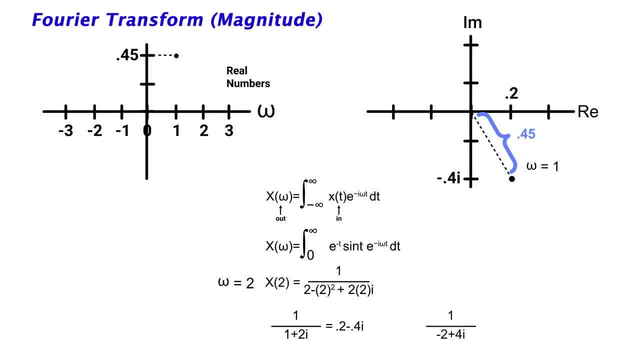 Now for omega equals two as the input. we get out one over negative two plus four i, which simplifies to negative 0.1 minus 0.2 i, and that will also go on the output graph. The magnitude for this is roughly 0.224, and that will also go on the magnitude plot for omega. 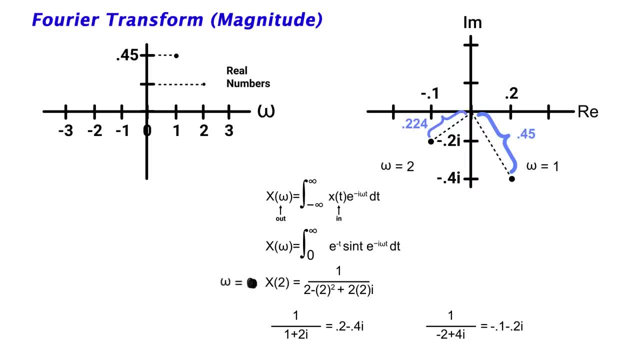 equals two. And lastly, I'll plug in, omega equals zero, which outputs just 0.5, no imaginary component, and that will also go on the magnitude plot. Remember that 0.5 is just the area under the curve of our original function, Well, accounting for the fact that areas below the x-axis are 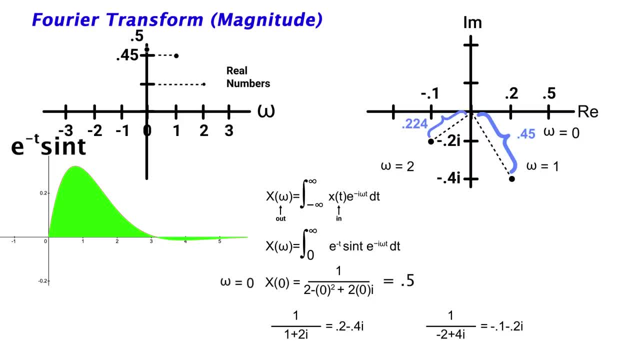 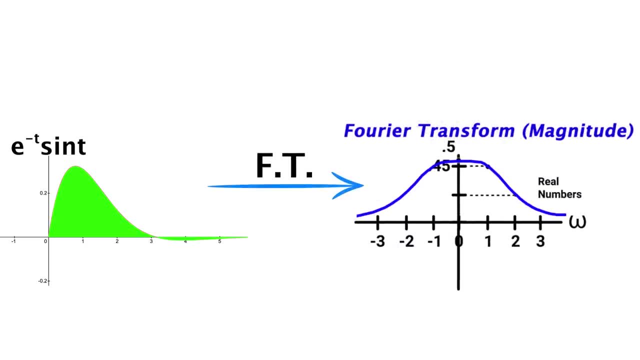 negative. If I were to plot all the magnitudes for any input omega, we'd get this: the magnitude of the Fourier transform. Keep this plot in mind because it will show up soon. but now let's get to the Laplace transform, so you can see just how similar it is to what we've done so far. 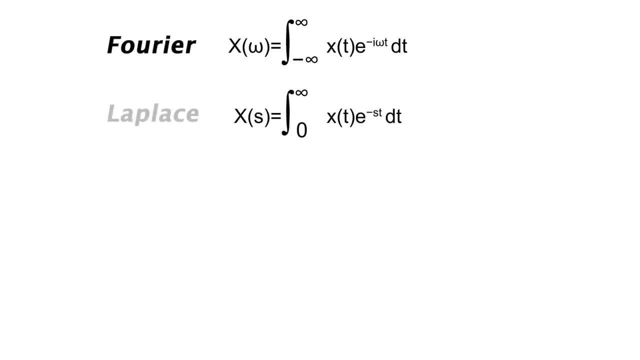 So here we have the Fourier transform again, and this is the Laplace transform, nearly identical. This could also be negative infinity, like above, by the way, but especially in engineering, we usually deal with signals that, like I said earlier, turn on at time equals zero, so we can analyze the transient response. 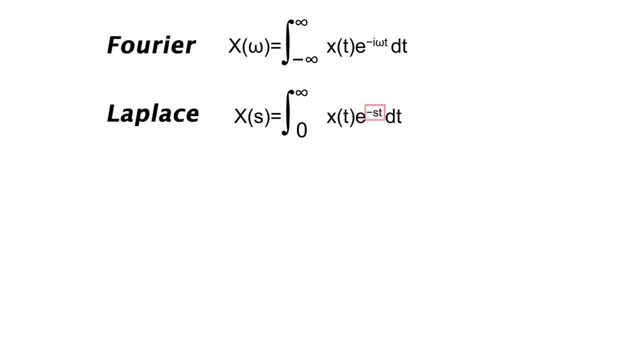 from there. The only other difference, though, is we have an s here instead of an i omega, But s is really alpha plus i omega, which I'll substitute in, because now we can separate that exponent into two terms. Now look at this: The Fourier transform. 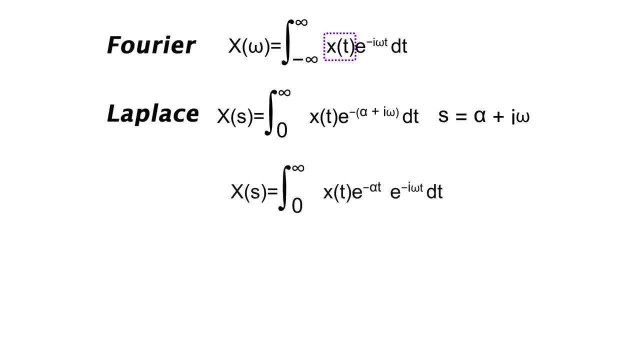 of something is found. by multiplying that function by e to the minus i omega t and integrating Well in the Laplace transform, we have the integral of something times e to the minus i omega t, meaning the Laplace transform of some function is just the Fourier transform. 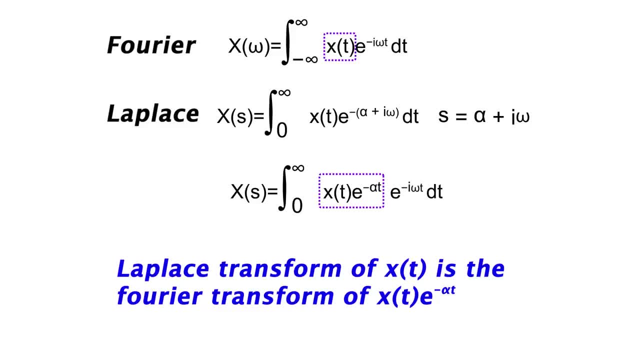 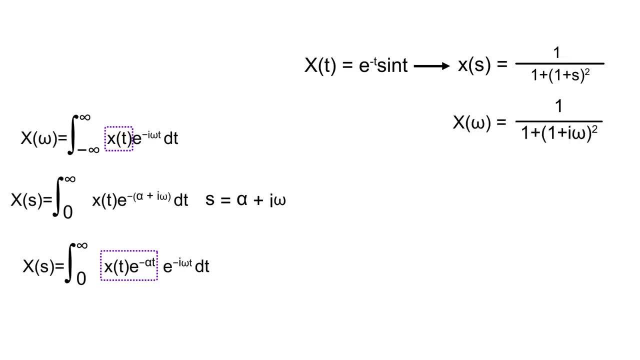 of that function times an exponential term. Doing this for all values of alpha, all real numbers, gives you the entire Laplace transform. To see what I mean by this, let's look at the Laplace transform of the same function. But it's nearly identical to the Fourier transform. The only difference is s represents a complex 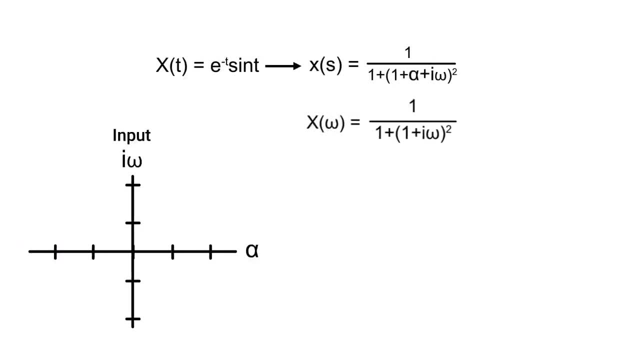 number, which means the input will require two dimensions: one for the real and one for the imaginary component. The output, just like before, will be complex. so we need four dimensions for the Laplace transform in total. But notice that when alpha is zero we get: 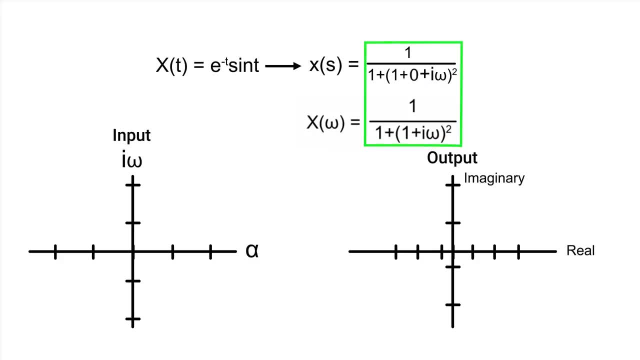 the exact same outputs as the Fourier transform. As in this alpha equals zero line, or the imaginary axis of the Laplace transform is the Fourier transform. Another way to see this is with the integral, because when alpha equals zero, the exponential goes to one and we're left with 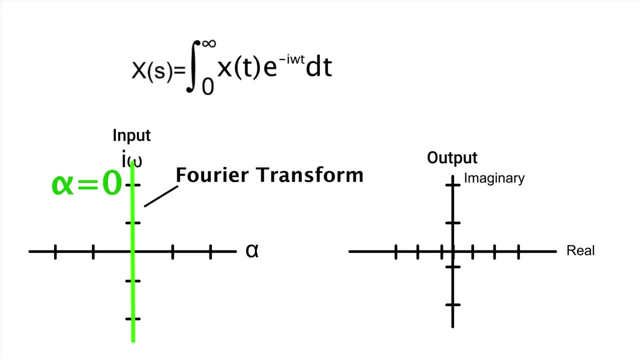 the original Fourier transform equation. So if I plug in something on that axis we should get the same magnitudes as before, Like if we put in zero for alpha and zero for omega, which goes here on the input, then out comes 0.5, that area under the curve which goes here on the output. And since I 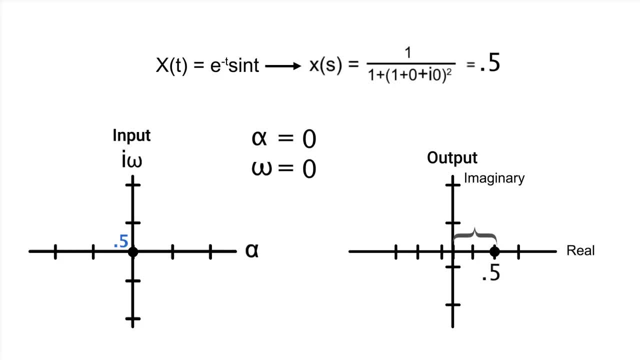 don't really have another dimension, I'll just write that magnitude above the corresponding input. If I plug in one for omega and zero for alpha, which is also on the same axis, then out comes the 0.2 minus 0.4i from before, which, on the output, is a magnitude of roughly 0.45.. And I won't show it. 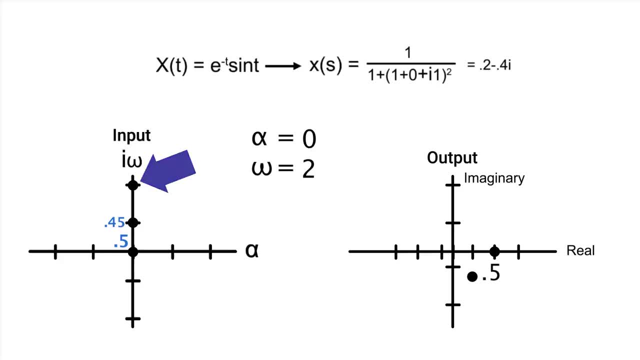 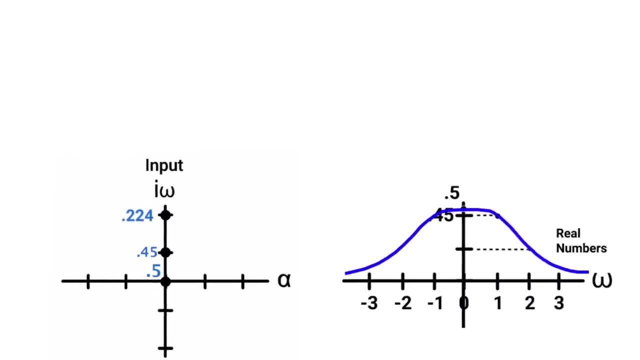 but if I did plug in this point where omega equals 2, the output would have a magnitude of about 0.224.. If I was using a third dimension to plot those magnitudes, then we'd see the exact same function on the imaginary axis. We could also make a contour plot though, Like just imagine looking down on. 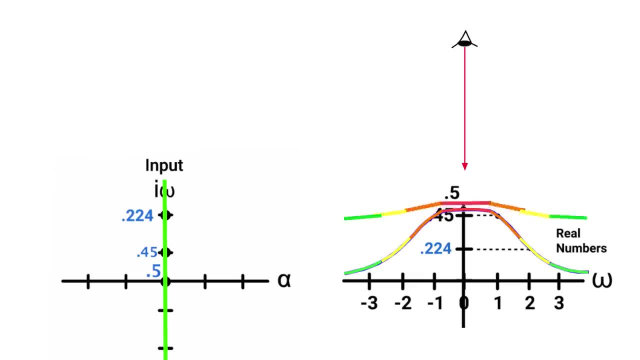 this graph where colors are assigned to different y values, because then those colors can represent the magnitudes. Then if I move the green line over to, let's say, alpha equals negative 0.5, the outputs will be the Fourier transform of something slightly different. Let me just put the original Laplace. 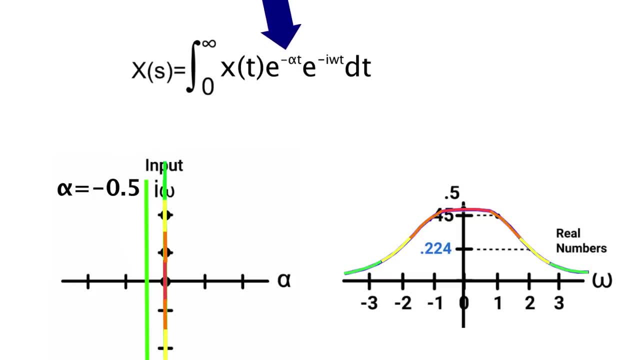 equation back up top and you'll note that since there's already a negative sign here when I plug it in, this will just calculate the Fourier transform of our original function times e to the positive 0.5t. That Fourier transform will look like this And again I could write the magnitudes to show the outputs: 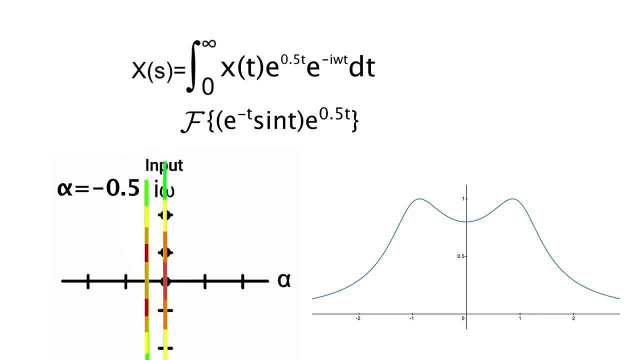 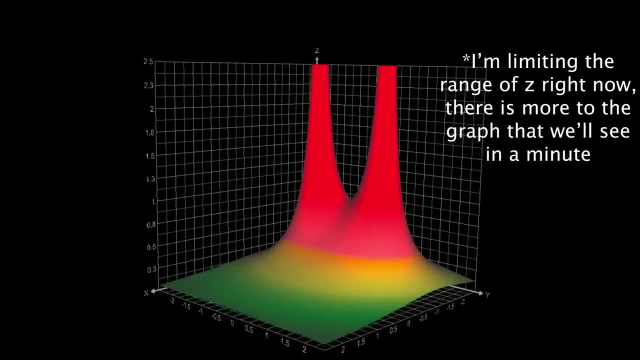 or I could use colors. If alpha is swept through the plane, we get the entire Laplace transform plot, And if we actually use a third dimension for those magnitudes, it would look like this: What I've shown in green- which I'll fade the plot a little so you can see- is all the inputs s. 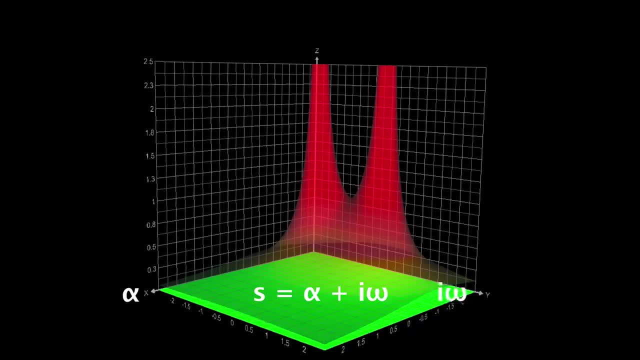 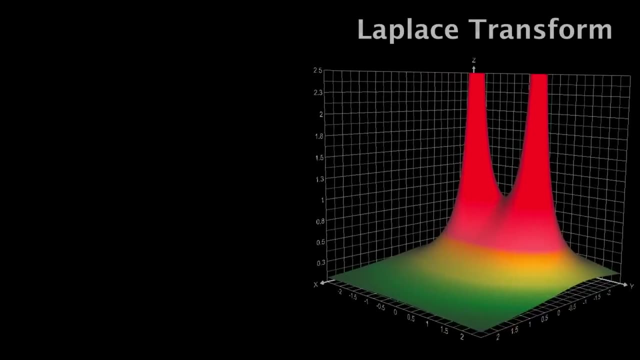 X represents alpha and y is really i omega. The 3D plot itself is the magnitude of the complex outputs. This is the Laplace transform of the original function e to the minus t sine of t. The thing is, this doesn't tell us much just by looking at it. So what I'm going to do is graph the equation. 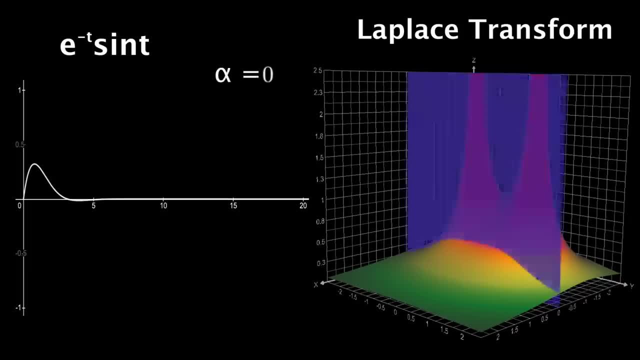 alpha or x equals 0, that'll give us a plane as shown, Because remember from before we had a plane that was a plane, And so we've got a plane. that's a plane, Because remember from before we had a plane that was a plane, And so we've got a plane. that's a plane. 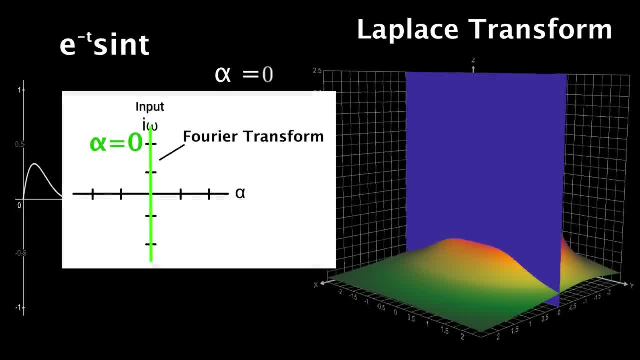 And so we've got a plane, that's a plane. And so we've got a plane, that's a plane, Because, remember from before, the alpha equals 0 line actually yields the Fourier transform of the original function, which we can see with the intersecting curve. 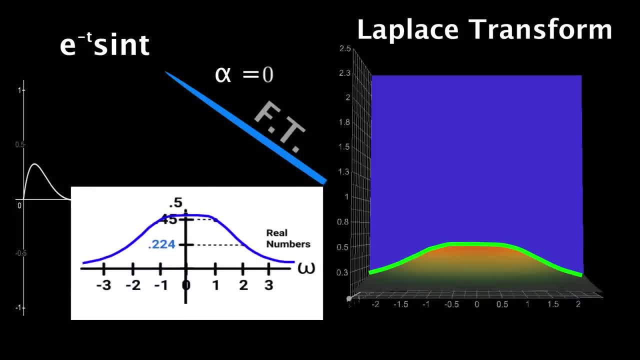 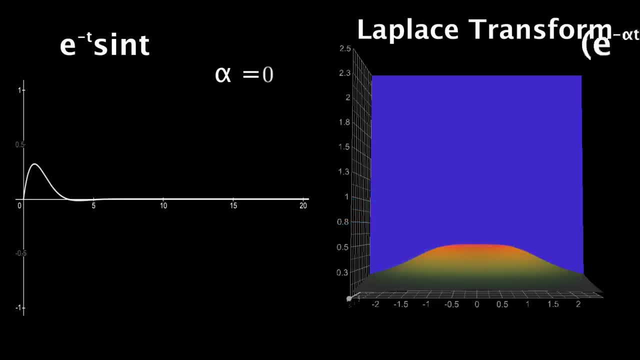 This is what I meant by the Fourier transform is a slice of the Laplace transform. But now I'm going to decrease alpha while also plotting the original function times e to the minus alpha t. Right now alpha is 0, so that exponential is just 1.. But as I sweep alpha we start to see both plots change. 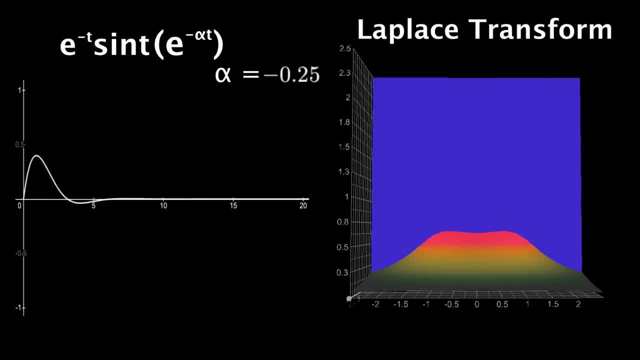 And what you're seeing with that intersection on the right is the Fourier transform of the plot on the left at any given time, Like here. I'll pause at alpha equals negative 0.5, because this is what we just saw a minute ago. 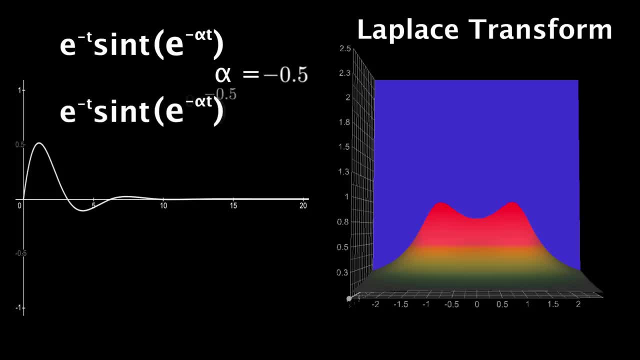 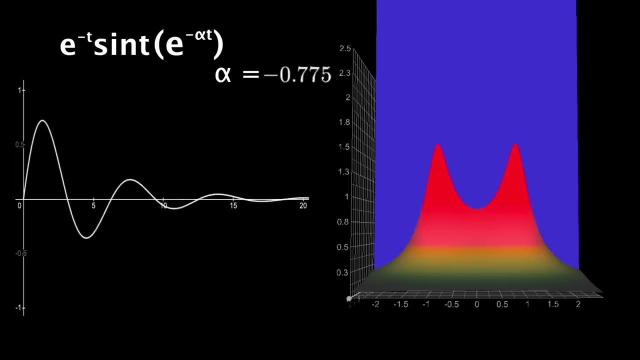 where the original curve times e to the positive 0.5t, because that double negative has a Fourier transform with those two small peaks. Then I'll extend the range of z, because as we get closer to alpha equals negative 1, we get an intersection with two much higher and narrower peaks where rendering also isn't looking so good. 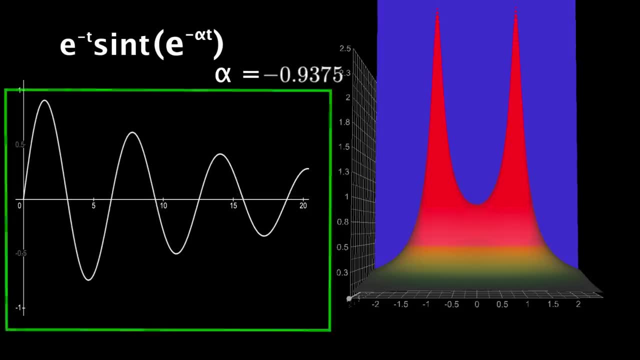 But anyways, this happens because the left plot is approaching just a regular sinusoid, since the exponentials are about to cancel once we get to alpha equals negative 1.. And we saw before that a pure sinusoid has a Fourier transform of two infinite spikes, which we can also see on the 3D plot. 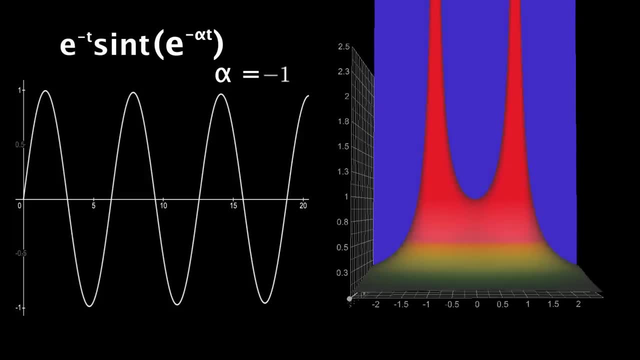 So the quick summary to what we've seen already is that to construct a Laplace transform, take whatever function you want to work with, multiply by e to the minus alpha t for some alpha. let's just change it to something random like negative 0.93,. 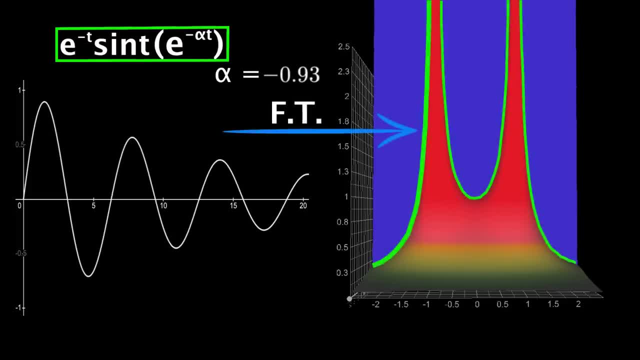 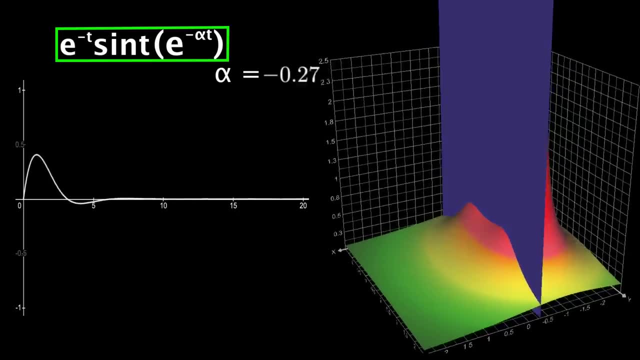 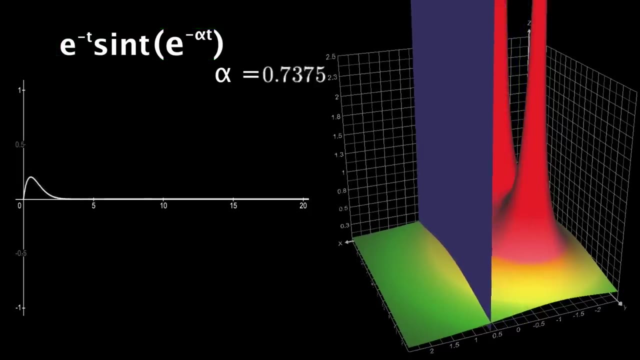 and graph the 2D Fourier transform of that function, Then keep doing that as you sweep through all values of alpha, stacking two-dimensional Fourier plots side-by-side, until you get your 3D Laplace transform. You will likely not be shown this in a classroom setting, and that's because most of it pretty much doesn't matter. 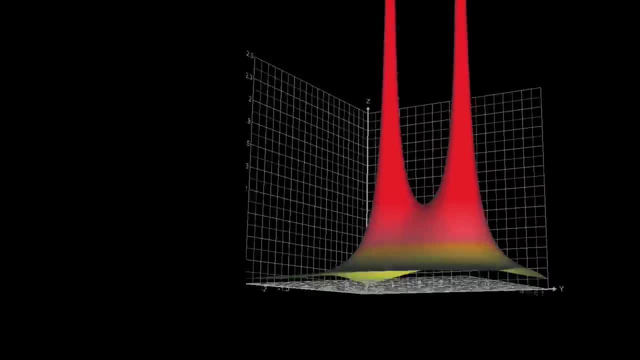 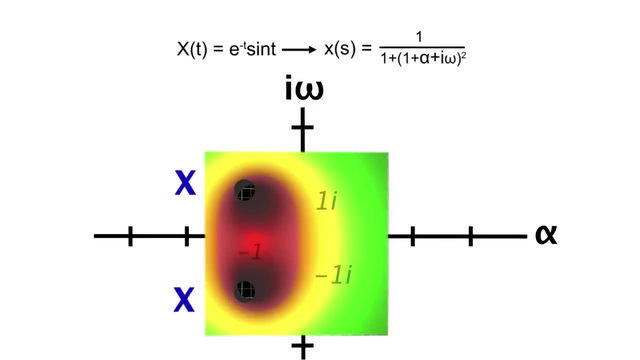 All we care about are these two peaks, which do not matter- They do go to infinity- known as the poles. Now, if we go back to the 2D plot, those poles are located at negative 1, plus and minus i. 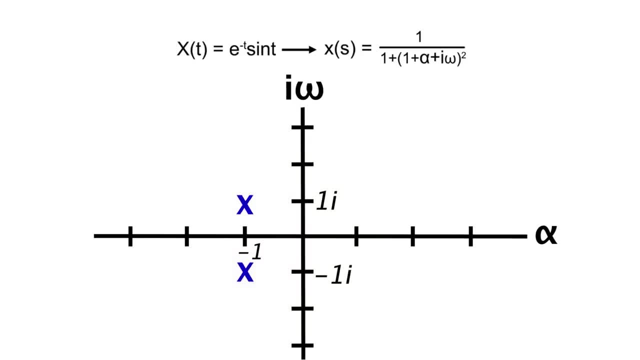 which we can represent with an x Poles, and also zeros, which doesn't apply to our function- are pretty much all you'll ever see for these plots. The reason the poles are there, though, is because, if we plug in negative 1 plus or minus i into the Laplace equation, 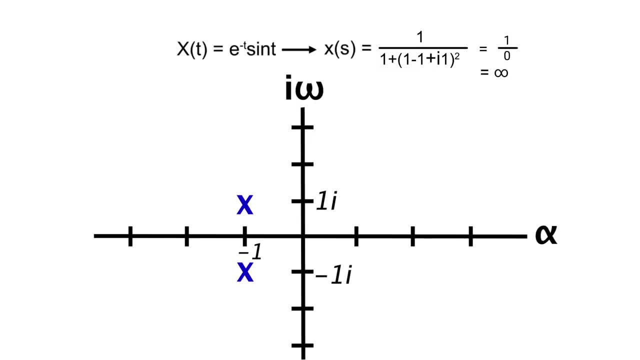 we get 1 over 0, which I'll just write as infinity, because on the plots those are represented with an x. Okay, And one more thing you'll notice: when I was sweeping the alpha plane, I stopped at those poles- or alpha equals negative 1, and never went behind that. 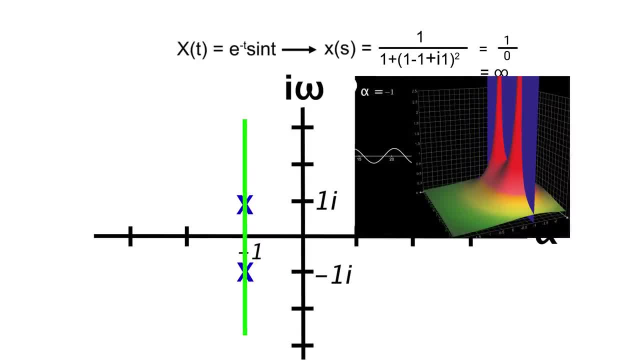 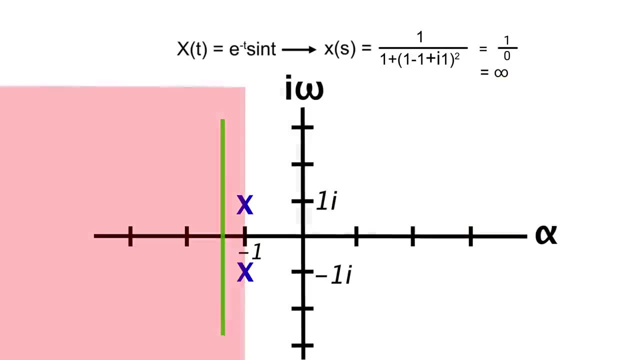 That's because once alpha goes below negative 1, the function we were plotting diverges, which means the Fourier transform of this does as well. So the Laplace transform doesn't actually exist in that region, whereas this is the good region which we give a name to: the region of convergence. 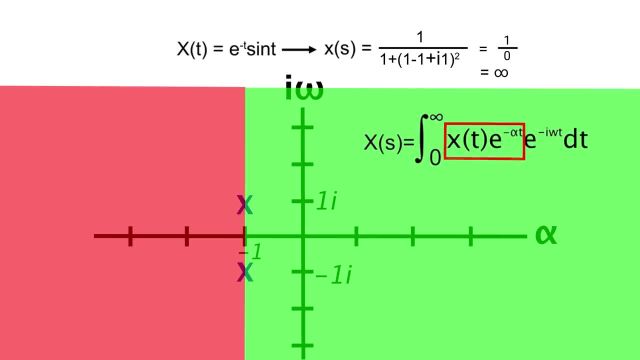 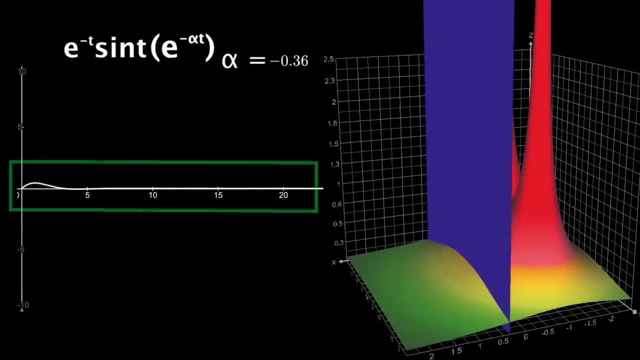 Just think of this region as all the alphas, such that this part of the Laplace transform eventually converges to zero. This means everything I said earlier with taking the Fourier transform of this function and that being a slice of our plot is true if that slice is in the region of convergence. 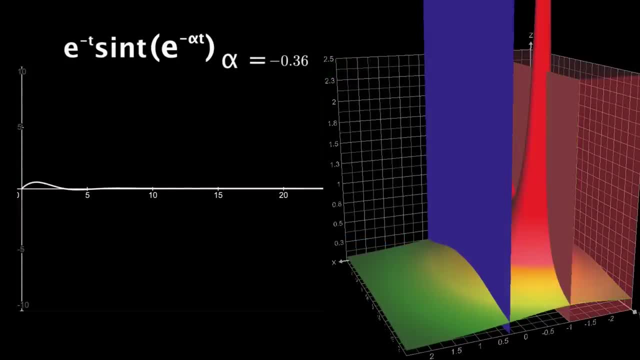 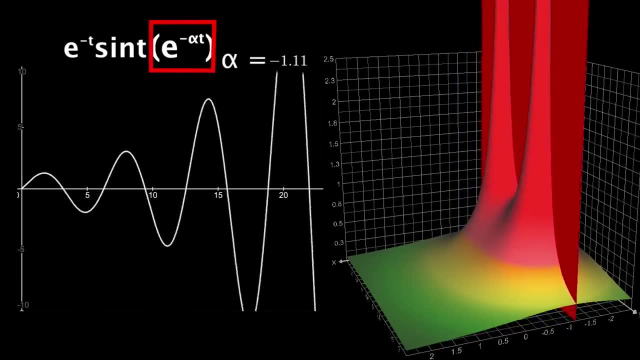 This part is so we're good there. However, this part is not, which is why, again, the function diverges for those alpha values. Essentially, this exponential term has now won, making Laplace undefined in that region. Anyways, going back, notice that for our pole, the imaginary coefficient of the Laplace transform is 1 over 0.. 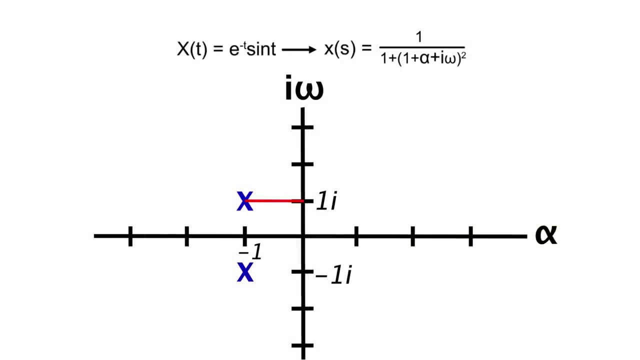 The imaginary coordinate is 1 and negative 1, which matches the coefficient or angular frequency of our sinusoid. The real component of negative 1 matches the coefficient in the exponential term. This is finally what the Laplace transform visually tells us. The imaginary axis represents the sinusoids and if my poles are on that axis, 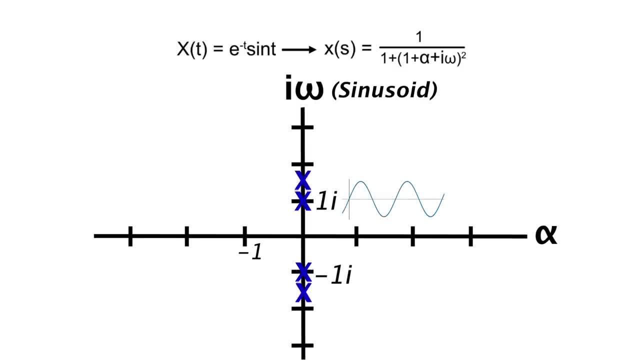 it means my original function is just sinusoidal, and the further from the origin the poles are, the higher frequency that signal is. If my poles are on the real axis, then they're only exponential- The exponentials in the original signal, which decay faster as we move further from the origin. 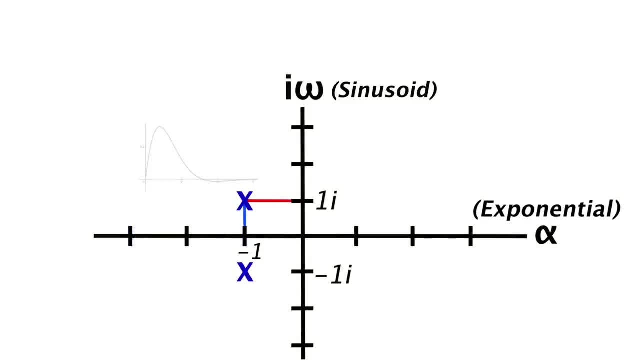 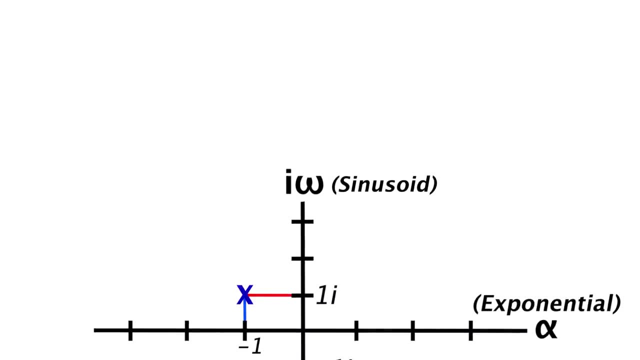 When the pole has real and imaginary components, like here, then we have a combination. Since this graph is symmetric about the real axis, I'm going to move it down and, to help with visualizations, I'm going to change the x-axis, so every tick mark is 0.2 units apart. 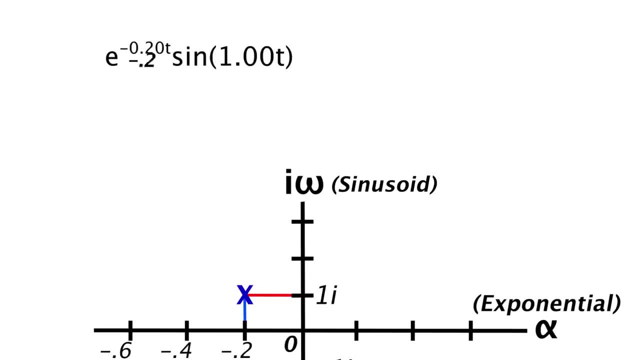 But anyways, now the pole represents this function with that exponential and sinusoidal component, whose graph looks like this: If I move the pole away from the x-axis, then the sinusoidal function is 0.2.. So the pole is now a real component and the exponential component is a sinusoidal component, whose graph looks like this: 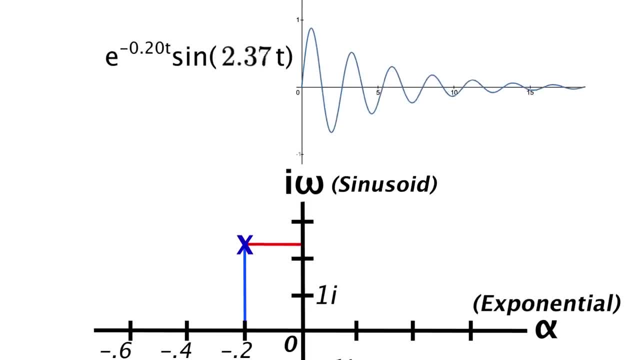 If I move the pole away from the x-axis, then the sinusoidal function is 0.2.. Then the sinusoidal frequency increases, causing faster oscillations, and the resulting equation will have an angular frequency that matches what we see on the imaginary axis. If I move to the left, then the number in the exponent gets more negative. 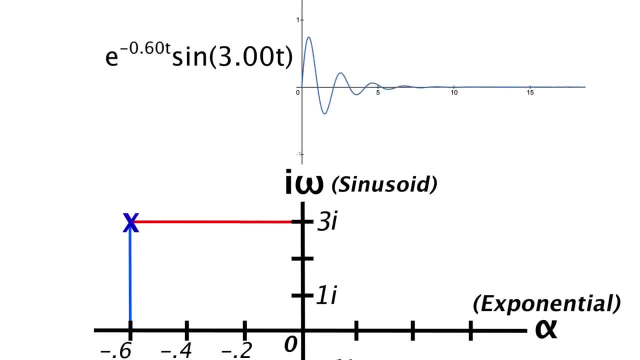 causing for a faster decay rate. The equation for this function still has coefficients that match what we see on the axes, And if I move to the right then the decay rate slows until we reach the imaginary axis where we get a pure sinusoid And poles on the right-hand side correspond to. 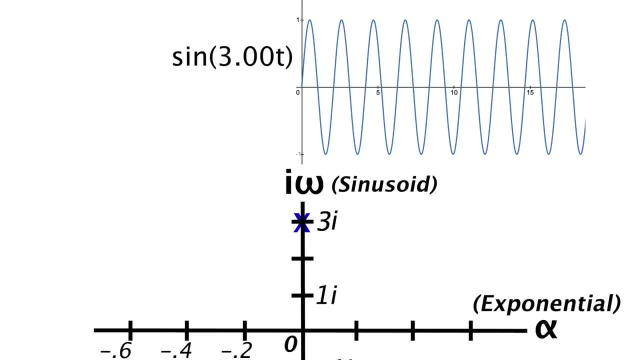 functions with exponential growth. If I move the pole away from the x-axis, then the exponential growth. So now Laplace transform equations should make way more sense. Like sine of 3t has a Laplace transform of 3 over s squared plus 9.. If we find the poles are on the denominator 0, we get plus. 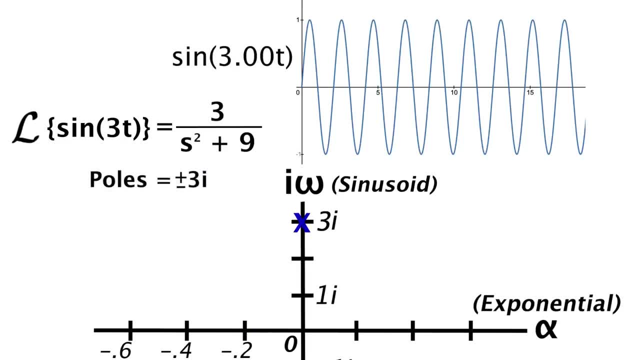 and minus 3i, and this tells us the original function has no exponential term, but it does have a sinusoid with an angular frequency of 3,, which we already knew. However, the most common talking point you hear with Laplace is not anything we've seen so far, but rather its ability to turn. 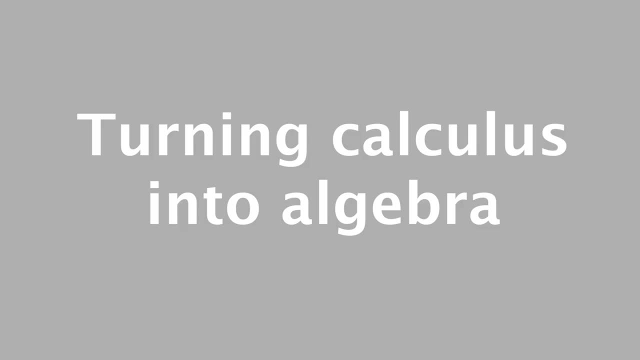 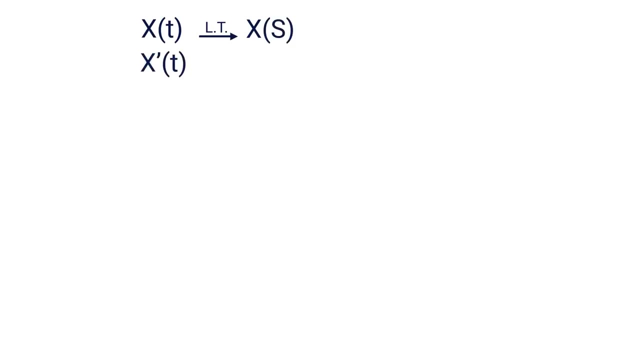 calculus into algebra. If we take some arbitrary function, x, it will have a corresponding Laplace transform x. But if you take the derivative of that same function, the Laplace transform will be the exact same thing times s. There is an extra term that has to do with initial. 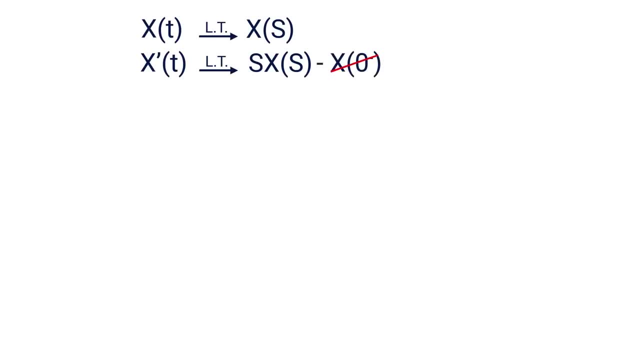 conditions, but I will assume those are 0 from here on. Then the Laplace transform of the second derivative is again the same x times s, squared this time, And some more initial condition terms that will ignore This pattern would continue, and this is where Laplace is really useful, For example this: 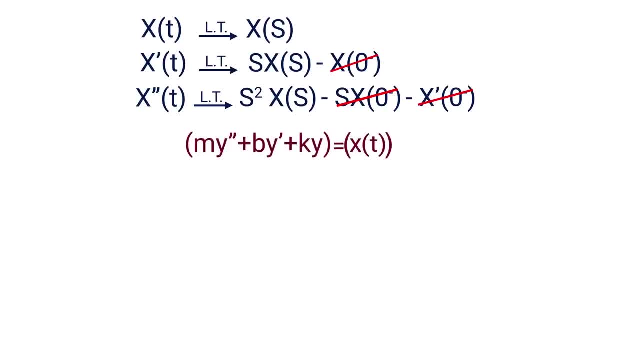 is the differential equation that describes a mass on a spring. We've got the force from the spring itself, the damping force, which is a multiple of velocity, some arbitrary input, x, and all forces sum to mass times, acceleration- here The grouping of the terms just came from. 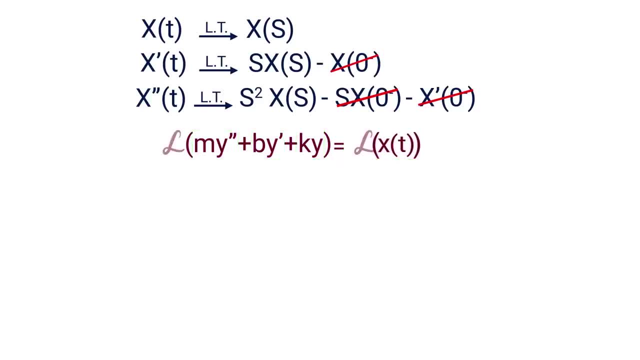 some rearranging. So what we can do is take the Laplace transform of both sides. However, due to linearity, this is the same as taking the Laplace transform of each individual term. The transform of some x is x, and for k times some y, it becomes k- y. 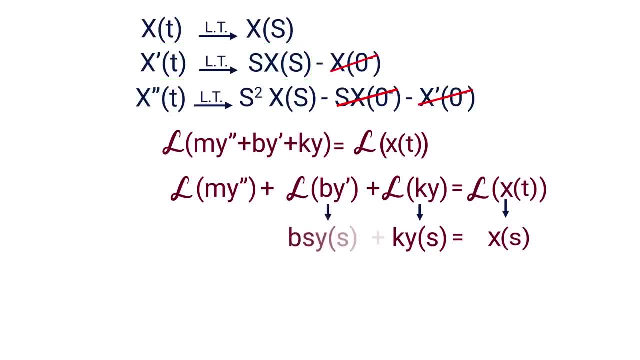 For b? y' from the rule above we get out the same y times s, and the b is there as well. Then the second derivative outputs m s squared y. Since all the terms on the left have a y, I can factor that out to get this here. Some of you may know this part as the auxiliary or 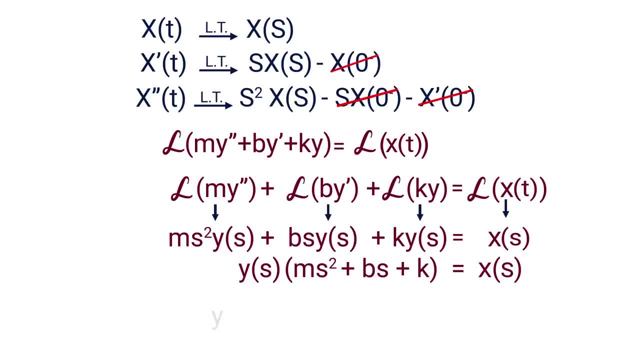 characteristic equation. We'll then isolate y and we're left with this here. So we may not know the actual output y, but, like we've already seen, if I know when the denominator of the Laplace transform is zero, aka the poles, then I can tell you a lot about. 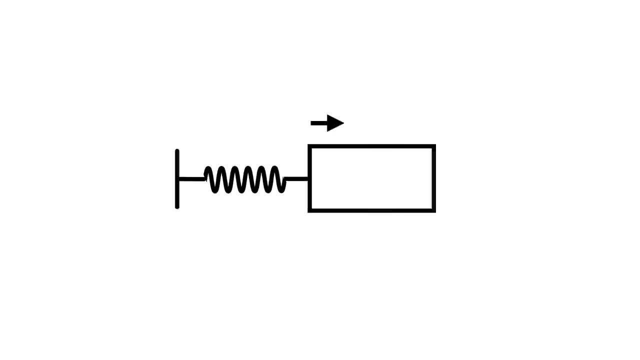 your output function. Let's assume the input is a constant force, because this is the same as having a vertical spring where the mass is subject to gravity. Like good engineers will say, the mass is one. thus force is ten newtons, And when the block is released, 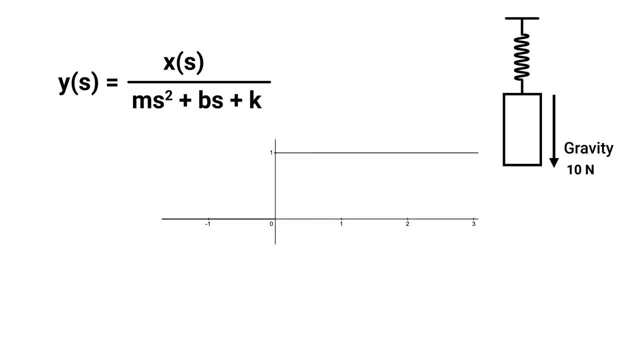 t equals zero, or the force is immediately turned on, so to speak. this is known as a step function. written u and its Laplace transform is one over s, Meaning our force 10u becomes 10 over s, which we'll plug in for x. Then again, mass is one. 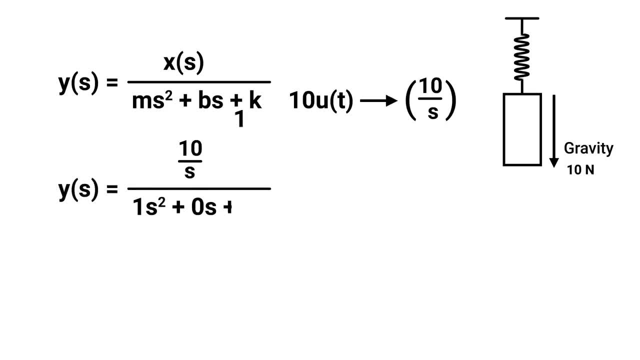 and let's say the damping coefficient is zero, while the spring constant is one, Then I'll just move the s down to the denominator. Since there's no damping, the spring will oscillate forever around in equilibrium. but let's check. this is showing an equation. 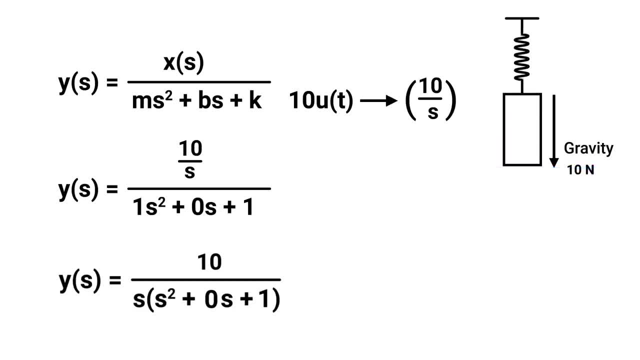 with our Laplace equation as well. We have one pole at positive i and another at negative i, which is what makes this part zero. Then we also have a pole at zero from the s out here, and we'll put everything on the pole zero plot. Again, I'm hiding the bottom to make room, but it 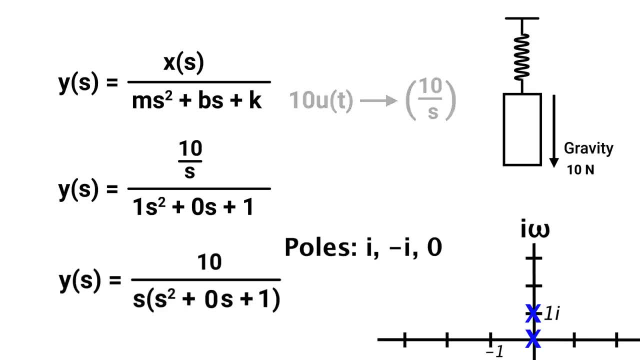 always looks identical to the top half, And now we have everything we need. These poles say that the output will have a sinusoid with an angular frequency of one, and we haven't seen a pole at the origin yet. but remember, this is the area under the curve. the intercept of the Fourier transform. 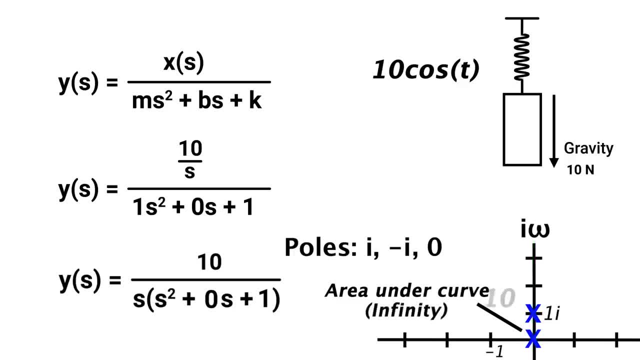 The pole thus represents an infinite area, which just means there's some offset in our output or something that doesn't converge to zero. to get that infinite area- Since we're considering the top to be y equals zero- then the output is exactly what we expected. If I increase the value of k or 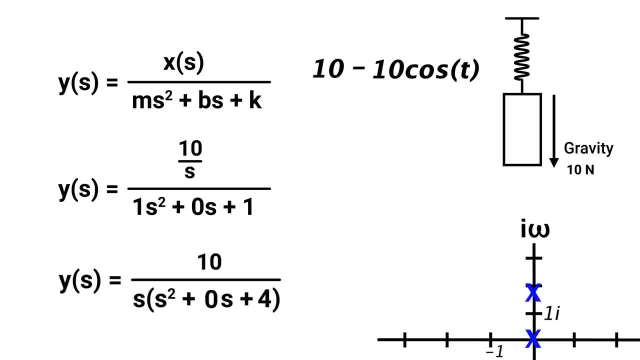 make the spring stronger, then the poles start to separate more and more, which represents faster oscillation. If I were to add some damping now or increase b, then we expect slow exponential decay. I'll just stop here- at b equals two, for example. so we can see there's now a sinusoidal and exponential. 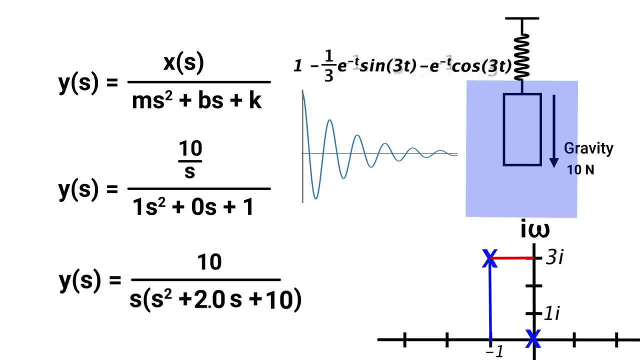 component to our equation which matches what was expected, even though, no, I'm not graphing the exact output. If we make the damping much stronger, we get to a point of critical damping where, finally, oscillations go up. If we make the damping much stronger, we get to a point of critical damping. 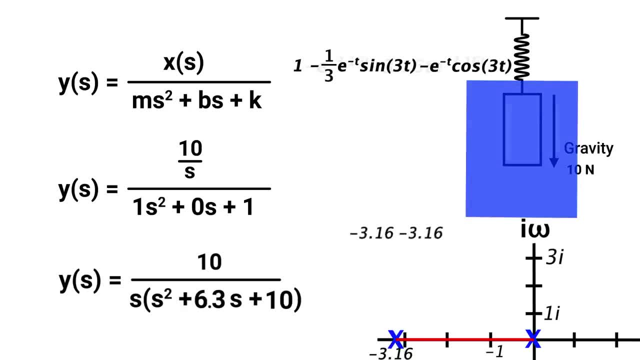 where finally, oscillations go up. If we make the damping much stronger, we get to a point of critical way and it's only exponential decay Then, moving from there, the exponential decay just slows down from this term not decaying as fast. Plotting the path those poles just took is the idea behind a root locus plot. by the way, for those in 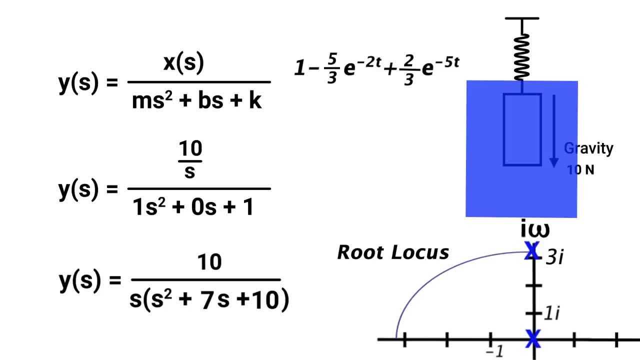 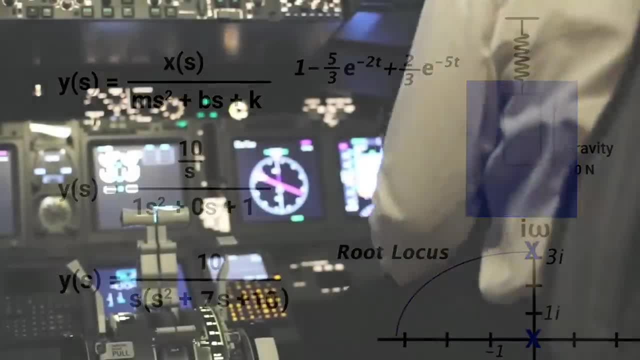 the controls class. but this is where the design part comes in, because by analyzing the locations of the poles we can determine how a system will respond to different inputs. Many systems out there would be extremely difficult with an applied data from melon graph, and yet they won't do. 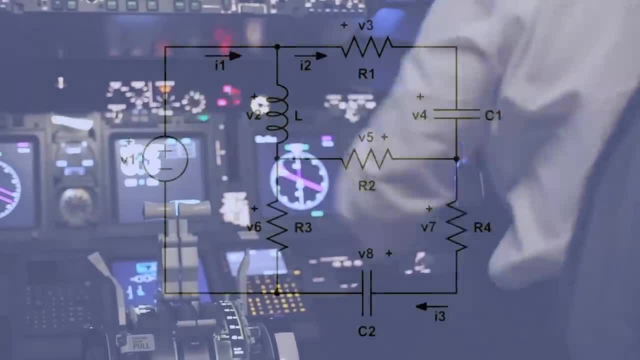 anything, because the rabbit isn't the only one we would require. They would create a motor that would difficult to solve using only functions of time. plenty of you probably know how not fun this would be to solve using only differential equations, but moving to the s domain makes it an algebra problem. 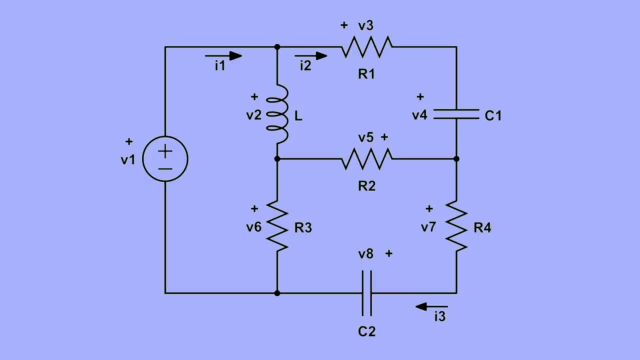 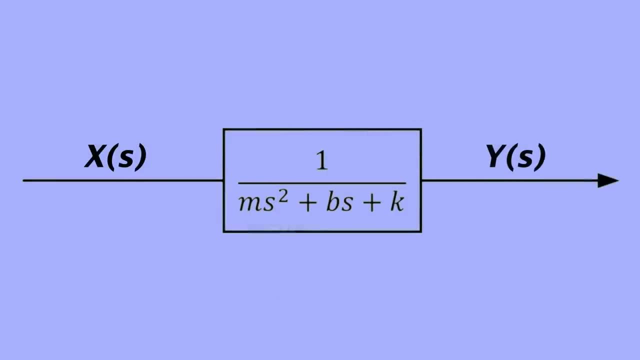 that's much more doable and especially in control systems, laplace is crucial. i mean, we just did a problem where an input was multiplied by the system's transfer function and we got the output transform. it wasn't that bad. but even when there's more going on between the input and output, it 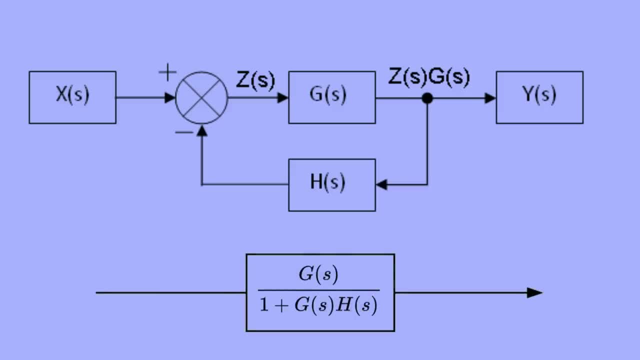 simplifies fairly nicely when using the s domain, as we can still just multiply the input by a more complex but still manageable transfer function to find the corresponding output. of course, there's plenty more to all this, and if you want to continue your learning, i highly recommend checking. 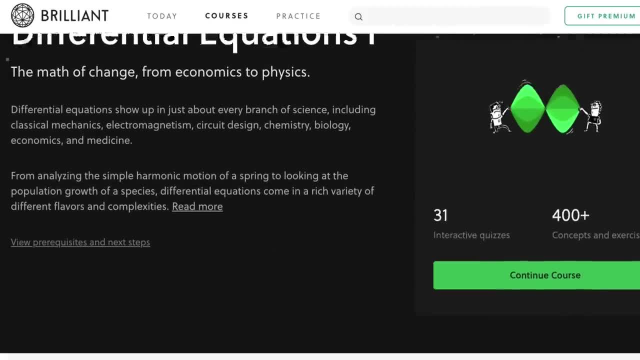 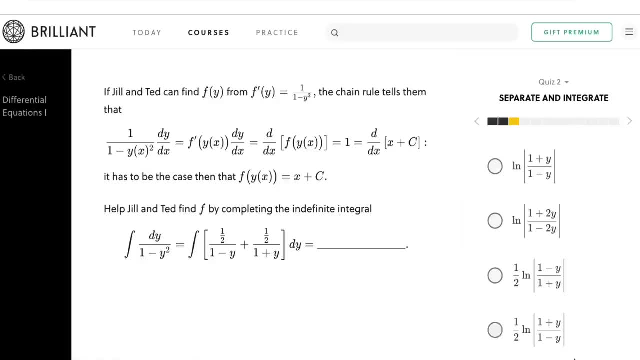 out brilliant series on differential equations. this includes two full courses which start at the basics for those who may need a refresher or just haven't learned this information yet, but by the second course they go through topics i never even came across in college as an engineer. so there's.